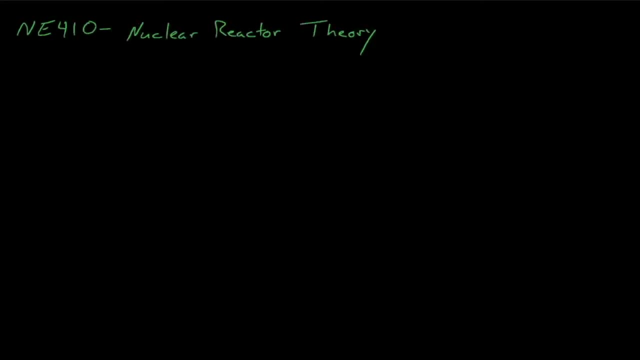 Hello everyone and welcome to the Nuclear Reactor Theory lecture series. This series will present lectures on material for an undergraduate or first-year graduate introductory course on nuclear reactor physics and radiation transport. At the risk of sounding humble, this course covers material that will serve as the foundation for your nuclear engineering education, and it is what. 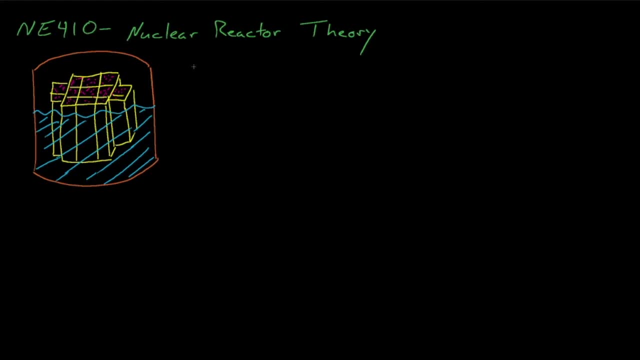 will separate you from other types of engineers. Other engineers may seek to model heat transfer or to predict the mechanics of materials, but nuclear engineers must do these things while also contending with modeling neutron shenanigans inside of a nuclear reactor- The main goal of this? 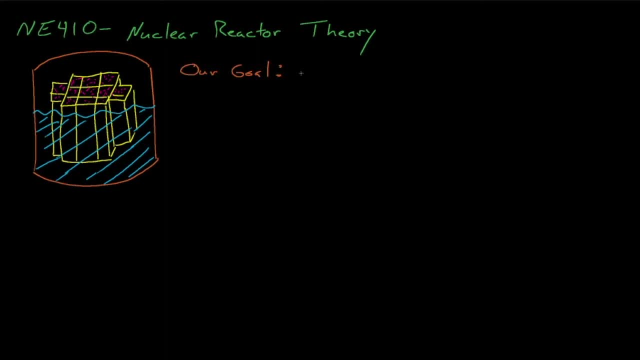 course is to develop methods to track the neutron economy of neutrons in a nuclear reactor. In other words, our goal is to estimate the criticality for these reactors. This will involve predicting how neutrons interact with various materials and fuels and computing neutron fluxes and reaction. 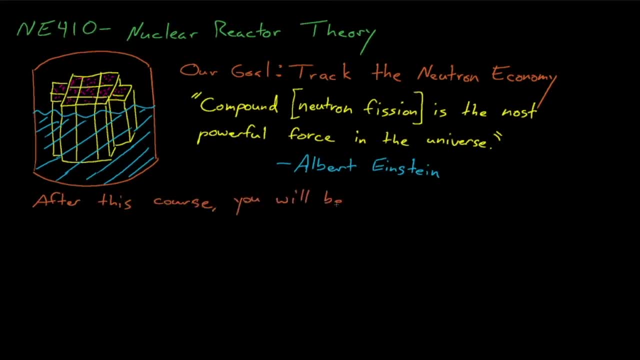 rates. After you complete this course, you will be prepared to take higher-level nuclear engineering courses in areas such as reactor design and fuel cycle analysis, radiation transport and shielding, transient safety analysis, isotope production and radiation effects on materials. Our educational goals for this course are summarized in our syllabus, but some more. 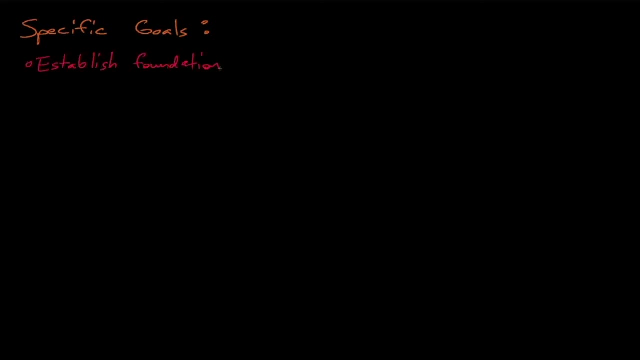 specific goals include establishing a foundation of nuclear engineering knowledge, modeling how neutrons interact with materials inside of a nuclear reactor and studying how neutrons interact with materials inside of a nuclear reactor. This course will also provide you with an opportunity to study how neutrons interact with materials inside of a reactor, which will include estimating. 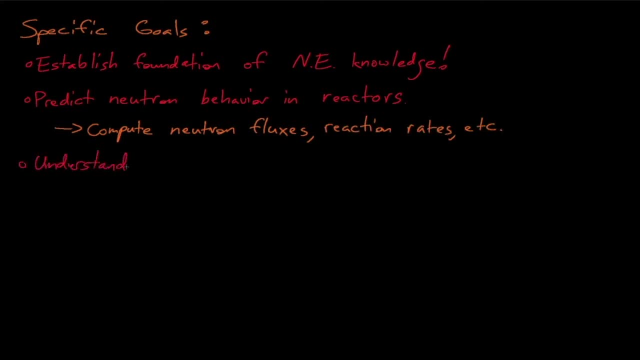 neutron fluxes and generating multigroup cross-sections. understanding basic nuclear physics concepts, including the physics of nuclear fission, moderation, radiation, transport, criticality, kinetics and homogenization. And, lastly, we'll try to understand basic reactor physics concepts. Ultimately, our 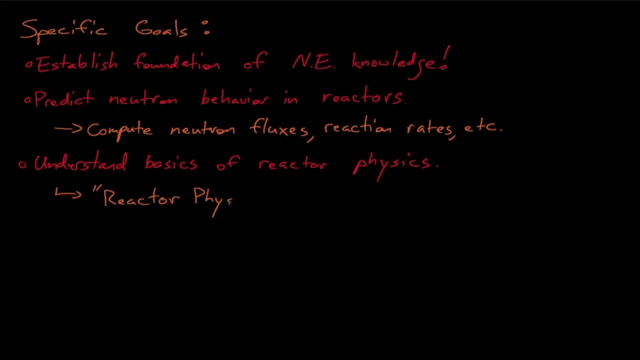 goal here is to establish a sort of reactor physicist's intuition, which will provide us with an innate intuition of how different changes in the reactor system will affect the reaction of the reactor. This will provide us with an innate intuition of how different changes in the reactor system 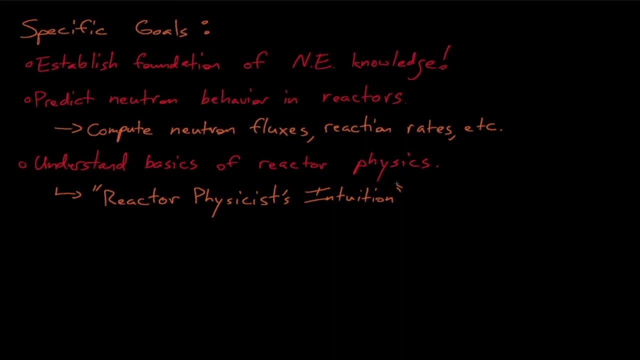 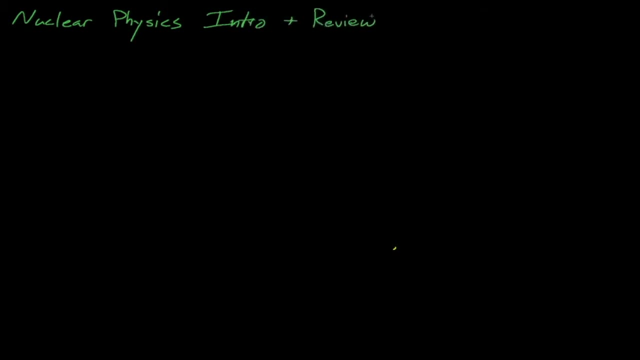 will impact neutron behavior inside of a reactor. Now, before we get into the real meat for this course, it's worthwhile to spend some time reviewing some basic nuclear physics concepts. You may already be familiar with much of this material, or it might be new to you if you're new to nuclear engineering. Either way, we 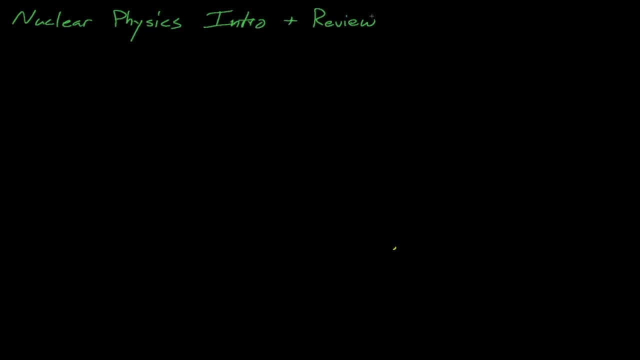 will build on many of these concepts later, so it's valuable to make sure that we have a solid foundation now. Our first topic to discuss is neutron cross-sections. Cross-sections are perhaps the most precise, persistent and most important concept in nuclear engineering, and they describe the probability. 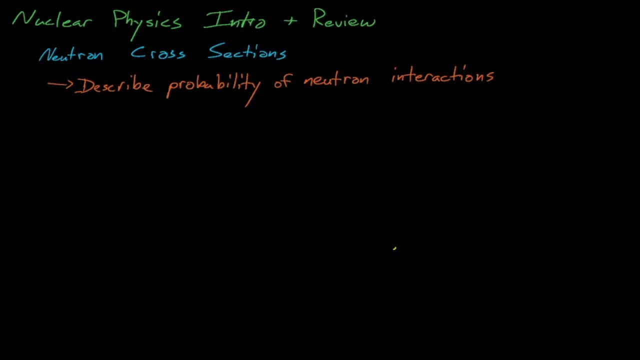 that neutrons will undergo some reaction within some region of space. Effectively, a nuclides cross-section describes the area that it presents to neutrons. Nuclides might have larger cross-sections if they're physically larger, but they could also have effectively larger cross-sections. 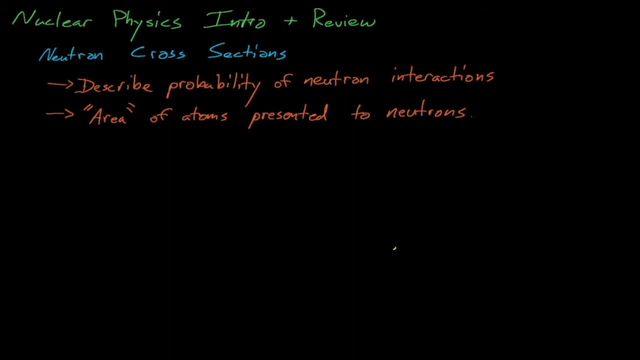 if they are more likely to interact with neutrons due to any kind of quantum physics trickery. Let's begin our discussion of nuclear physics by looking at the following two concepts. The first is the concept of nuclear physics. Nuclear physics is a concept of nuclear engineering. 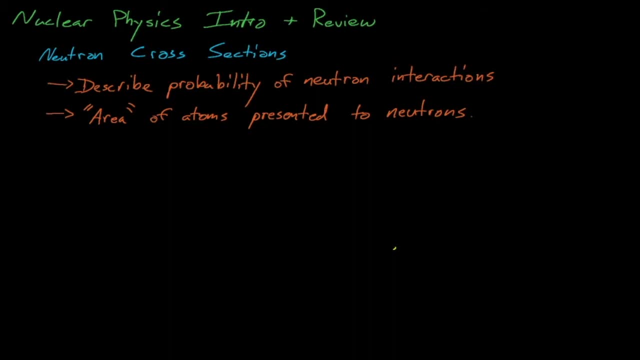 by using the concept of nuclear cross-sections to derive the uncollided flux in some media and to predict the mean free path of uncollided neutrons. Consider some flux of particles as instant on a chunk of material containing these round nuclei. The number of uncollided 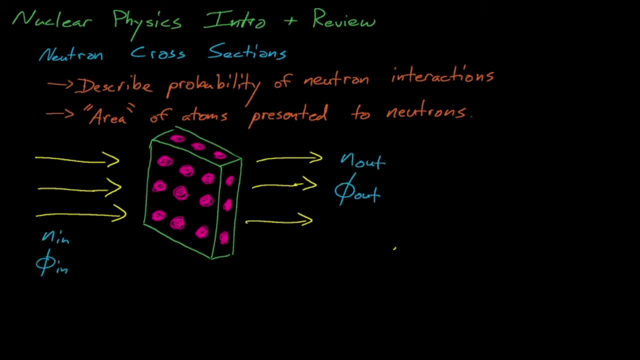 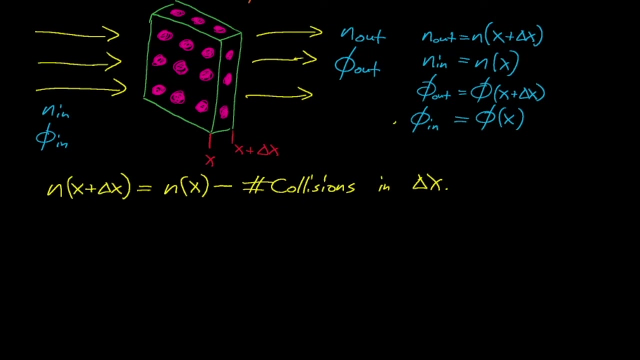 neutrons n that emerges out of this material at some x plus delta x is equal to the instant neutron population at x minus the total number of collisions suffered in the material. If we recall our definition of the microscopic cross-section as the area of these nuclei. 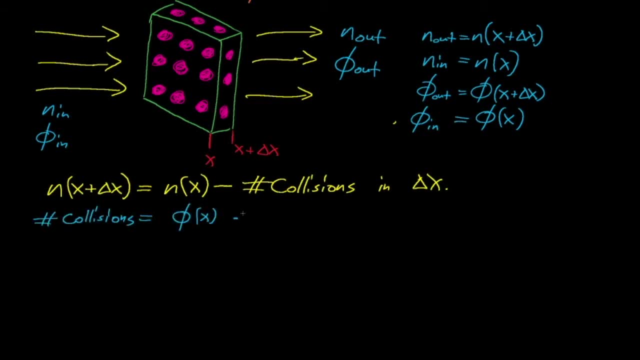 then this number of collisions in our thin slab is equal to the flux of particles which is, per unit area, instant on the slab times, the area of each target nucleus, which is, again, the cross-section times the number of nuclei present in our delta x thick slab. 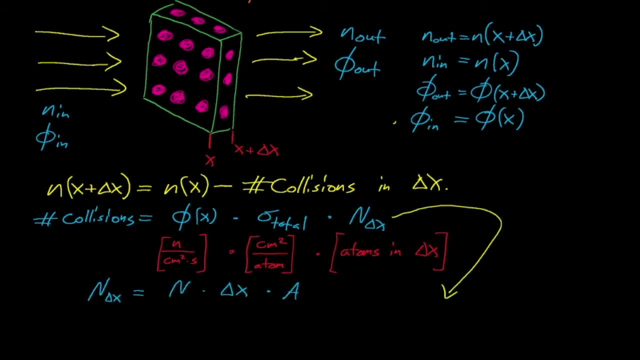 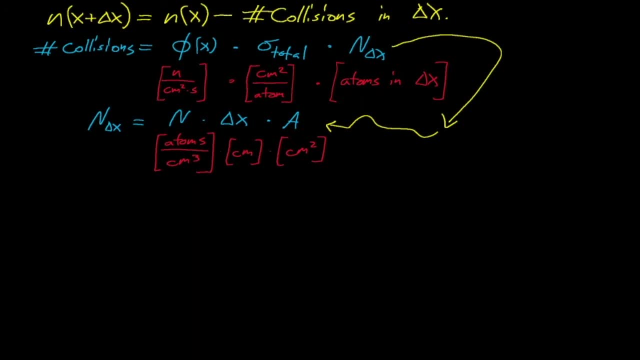 The number of nuclei present in this slab equals the number: density of nuclei in this material times. the thickness of this material times the density of the area in which the times the thickness of our slab times the area of our slab, Noting that the flux is equal to the rate at which particles are instant on. 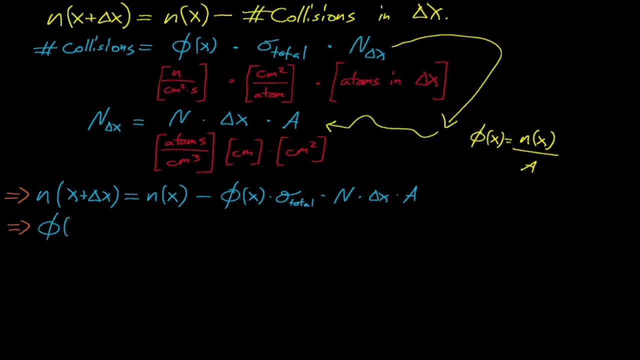 our slab per unit area. we can simplify this expression by dividing both sides by the area of the slab to convert n to phi. This conversion is helpful because in general it is much more useful to represent our neutron population using the neutron flux. 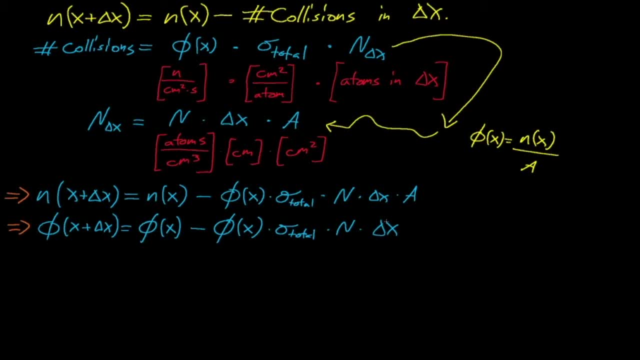 which does not depend on the area of the surfaces through which the particles stream. We will discuss these terms and how to convert between the terms much more formally and in much more detail later on in this course. From here, we can add in a dash of: 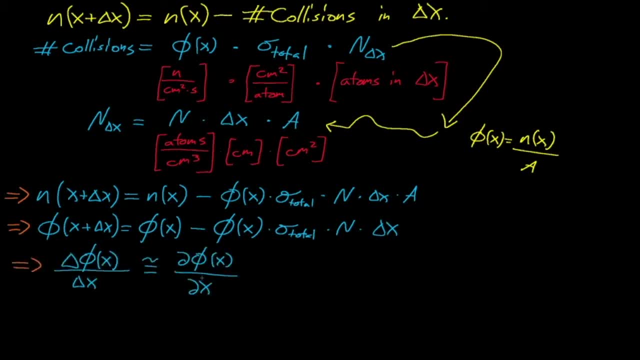 calculus to convert our differential fluxes and delta x in our slab to the derivative of the flux as a function of x, as shown here, and then we can recall our definition of the macroscopic cross-section to simplify this expression further. Lastly, we can solve this differential equation to find that the uncollided flux 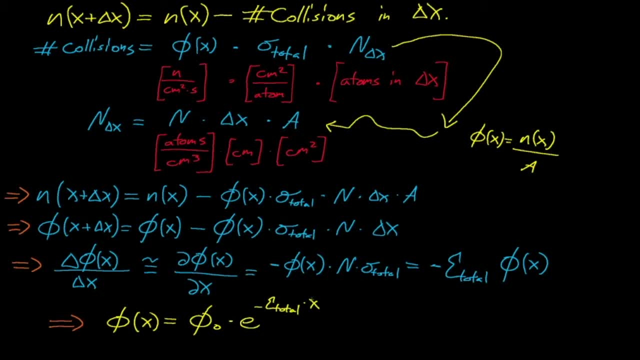 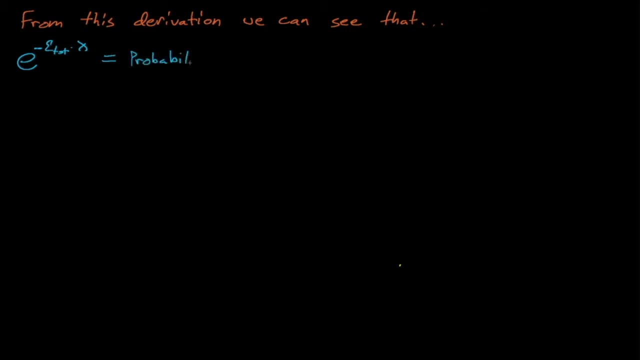 in a homogeneous slab is described by this decreasing exponential function. With this we can define the mean free path of neutrons in the material. but first let's talk about probabilities. We can examine our previous derivation to find that e to the negative sigma total times x. 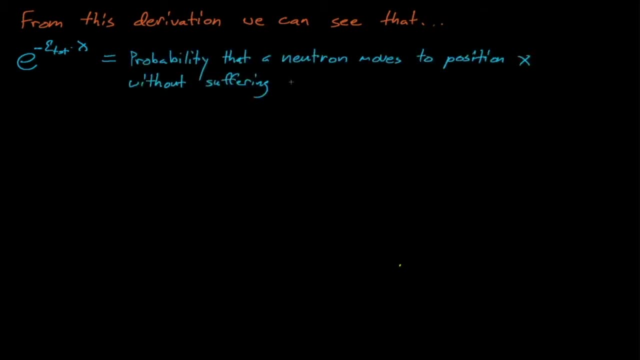 equals the probability that a neutron will move to position x without having a collision. Similarly, since sigma total times delta x is the probability that a neutron will be absorbed in some small delta x. we can develop a second term, shown here. that is actually the probability distribution that describes the 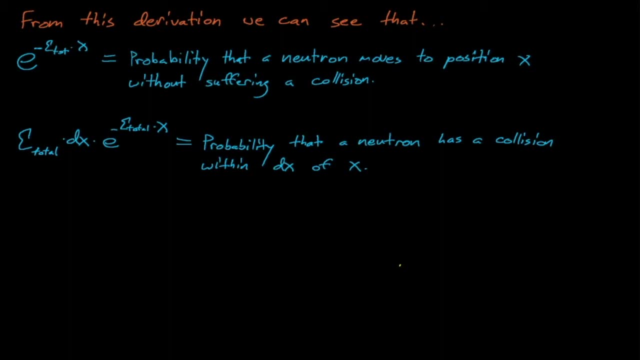 probability that a neutron will reach some location, x, and have a collision within delta x of x. As a probability distribution, this term has several properties, the first being that it is normalized, which is another way of saying that this term, when integrated over all bounds. 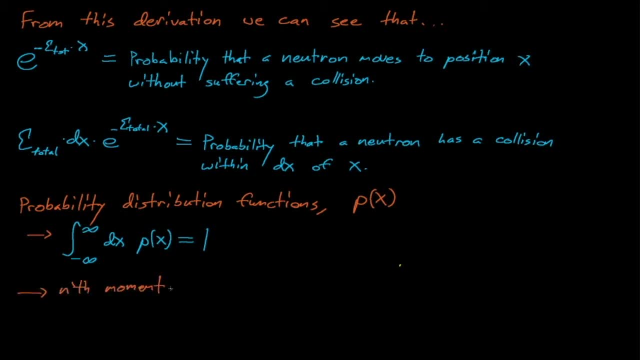 will equal 1.. Second, we can calculate the moments of this probability distribution by multiplying it by some x to some power of n, and then integrating it over all bounds. This term will give us the nth moment of x, The average x described by this probability. 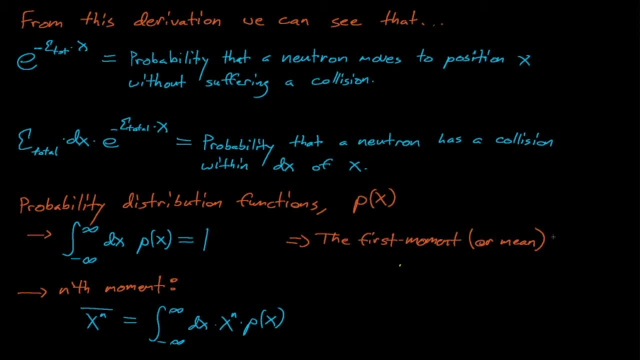 distribution is equal to the mean, which is also equal to the ratio of the first and zeroth moments of our probability distribution. Again, here the zeroth moment equals 1, via the definition of a probability distribution here, which gives us that the mean is simply described: 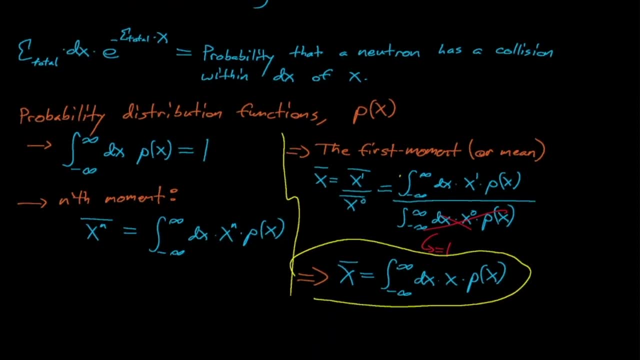 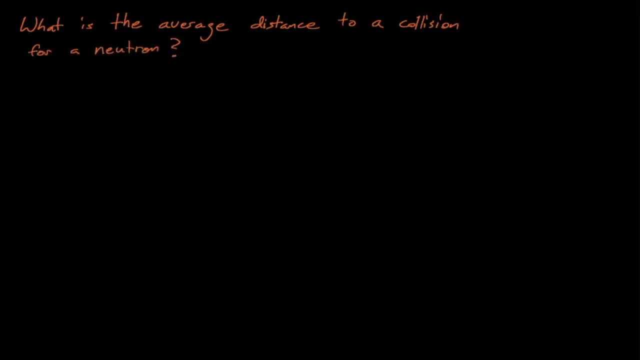 by this integration. Getting back into nuclear physics mode, it may be convenient to know the average distance that a neutron travels before suffering a collision. This term is known as the neutron's mean free path. From our discussion of probabilities, we know that the mean free path 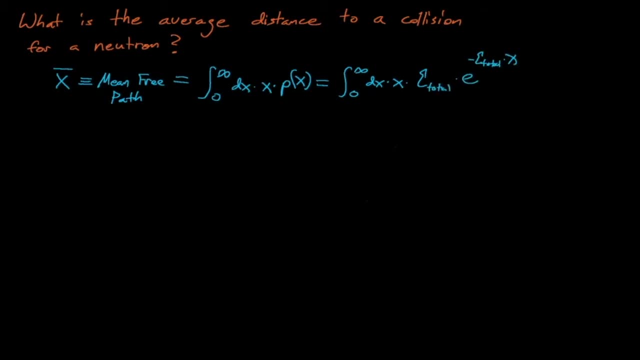 for a neutron is equivalent to the first moment of the neutron's collision probability distribution, which equals the integral from zero to infinity. with respect to x of x times sigma total times e to the negative sigma total times x, The bounds of this integral go from zero to infinity instead. 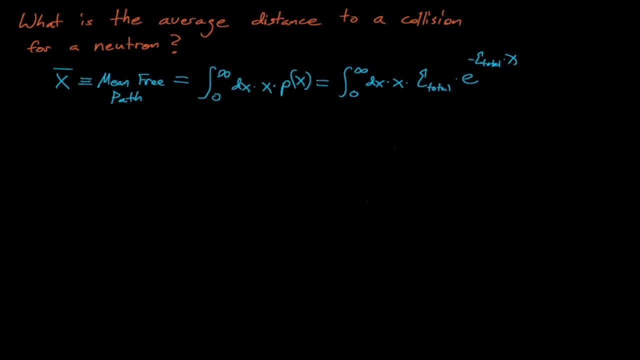 of from negative infinity to positive infinity, because it's impossible for our neutrons to have interactions before they actually reach our material. We can solve this integral using integration by parts, and after a fair bit of simplification, we see that the neutron's mean 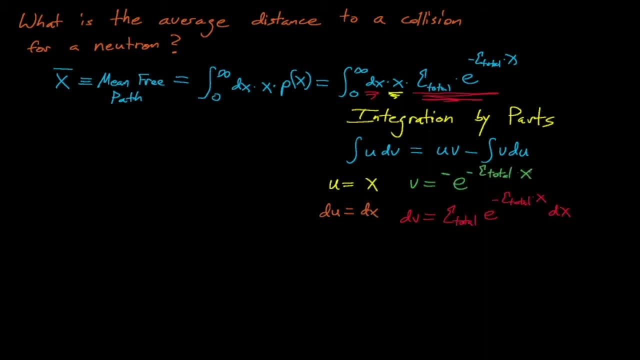 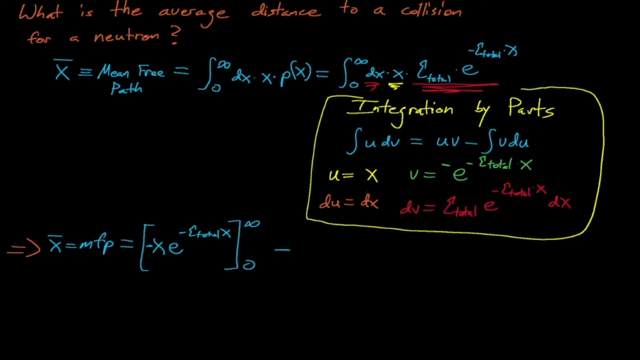 free path equals one divided by sigma total. You probably knew this before seeing this derivation, but being able to derive this is useful. It's also worth noting that this derivation of the equation assumes that we have mono-energetic neutrons, and later in this course we'll see. 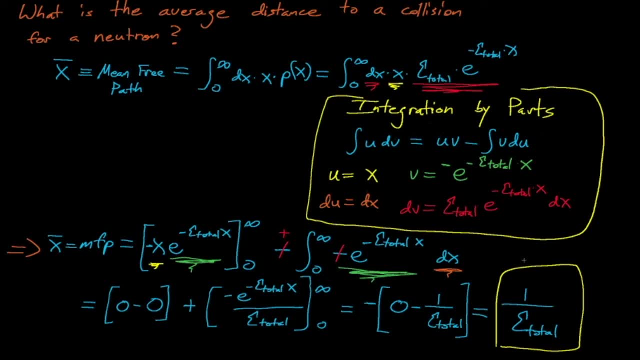 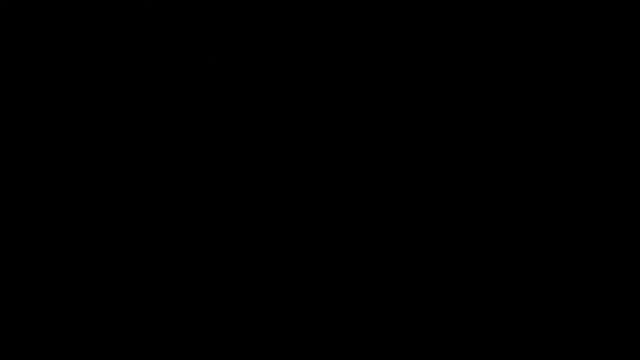 exactly how a neutron's mean free path will vary with its energy, and we'll also see the profound effects that this has on the neutron distribution in a system. In this course we'll discuss the physics of several kinds of reactions that neutrons can have with matter. so now it's worth. 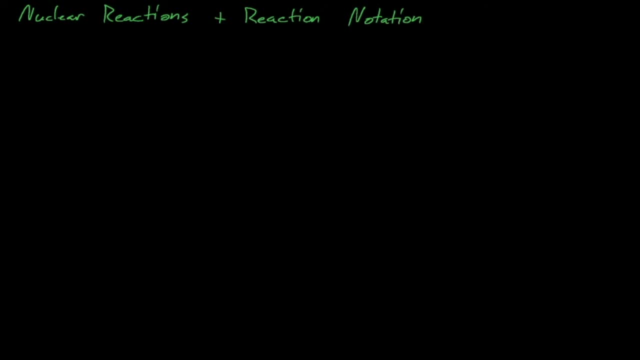 quickly discussing some common notation for reactions, as well as listing the most common nuclear reactions that we will encounter. This ECD notation is the common notation for describing a reaction where an instant particle B collides with the target nucleus A and produces the final or daughter nucleus D. 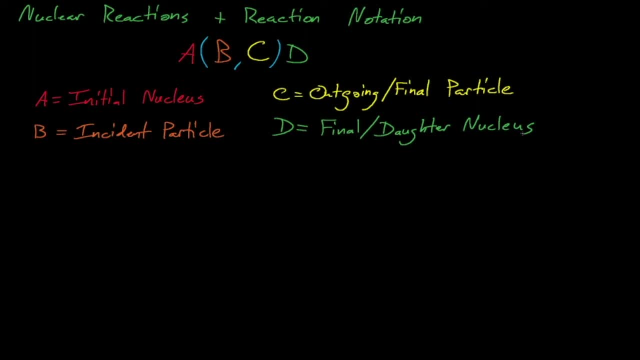 while emitting some particle or form of radiation C. For example, this is how we would use this notation to represent an alpha-n reaction with beryllium-9.. Here an alpha particle collides with beryllium, which creates a compound nucleus. 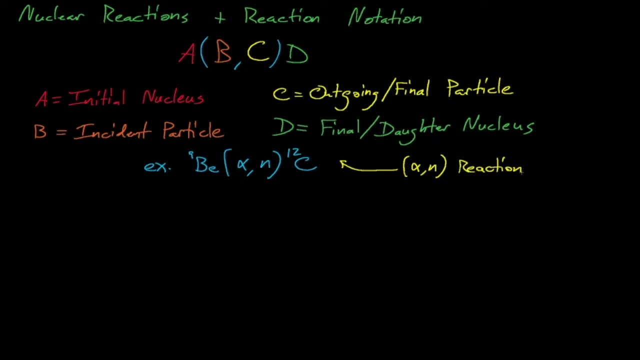 that then emits a neutron, resulting in a final carbon-12 daughter nucleus. This reaction is particularly important in nuclear engineering applications, as it is a common way to create a neutron source. What we can do is pair radioactive alpha-emitting particles with beryllium, which causes them to undergo this alpha-n reaction. 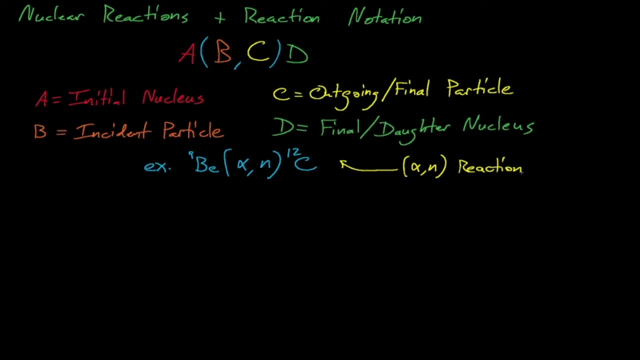 and emit neutrons. Both alpha emitters and beryllium are relatively plentiful and are safe enough to be handed individually, although beryllium can be quite nasty, which means that they allow for a relatively convenient source of neutrons. when combined, It's much more convenient than carrying around a 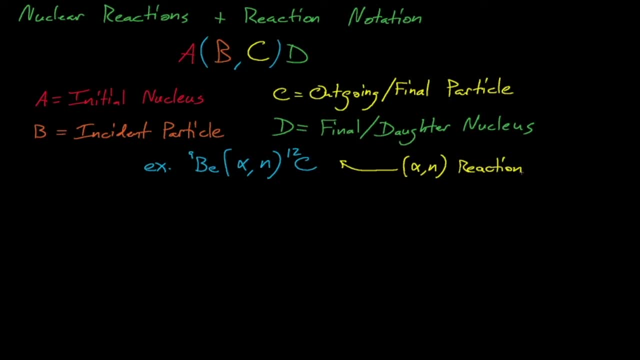 reactor in your back pocket. You will likely encounter beryllium-based neutron sources later on in your nuclear engineering lab courses. The amount of energy Q released by any reaction is equal to the sum of the masses of the reaction's initial particles in nuclei minus the sum of the masses of its final 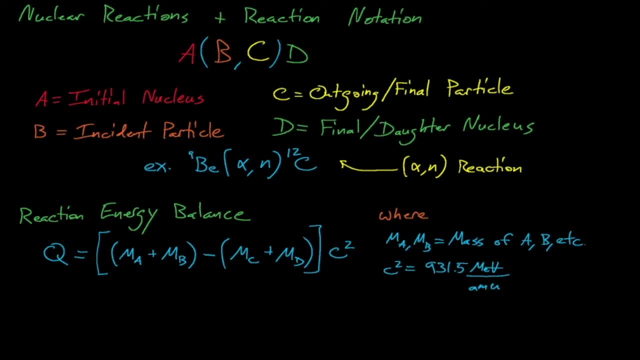 particles in nuclei All times c-squared, where c is the speed of light, which also approximately equals 931.5 MeV per amu or atomic mass unit. When looking up these masses to do these kinds of calculations, I find that the Cary website is very, very. 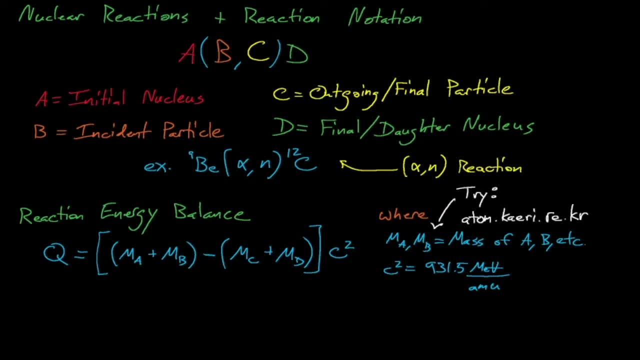 convenient, but you can feel free to use whatever source you prefer. If our Q value is greater than 0,, then this means that the reaction is exothermic, and if Q is less than 0, then the reaction is endothermic. 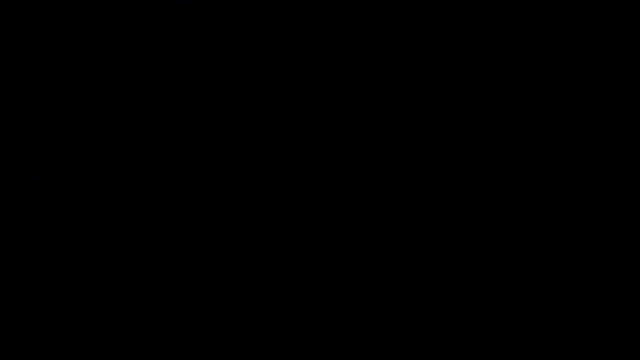 For example, consider the deuterium- tritium fission reaction, otherwise known as DT fusion. If we know the mass of the reactants and the sum of the masses of the products, then we can compute the Q value for this reaction which we find. 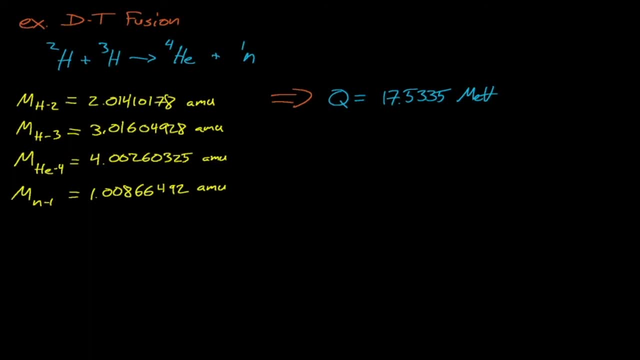 equals 17.5335 MeV. The almighty god of references. Wikipedia states that the Q value for DT fusion is 17.6 MeV, which means that our calculation, which ignore the initial kinetic energy of our reactants, was fairly on target. So what kind of. 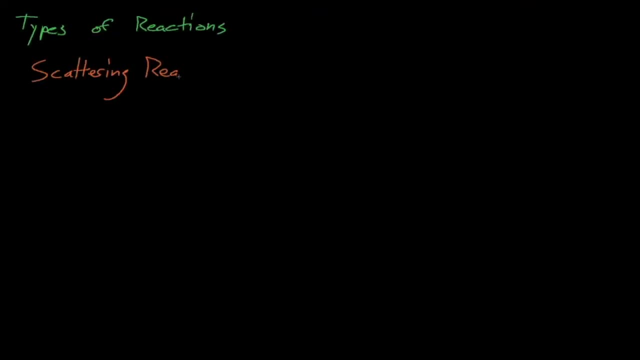 reactions can a neutron have with a nucleus? Generally, there are two classes of reactions to consider: scattering reactions and absorption reactions. Scattering reactions generally assume that a neutron bounces off a nucleus and is deflected into a new direction and perhaps into a new energy In general, 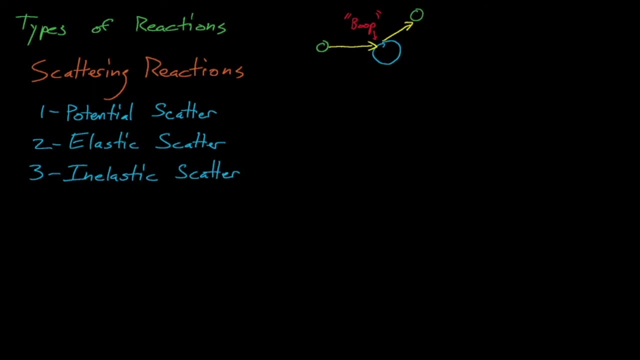 there are three types of possible scattering reactions to discuss: potential scatter, elastic scatter and inelastic scatter. For a potential scattering reaction: the neutron bounces off of the nucleus's potential energy well, much like a billiard ball bouncing off of another ball. The neutron doesn't. 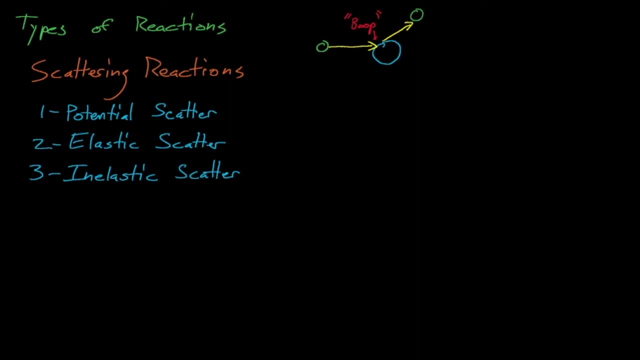 penetrate the nucleus's nuclear surface and thus kinetic energy is conserved. during this interaction, During elastic scattering, the neutron does in fact penetrate the nuclear surface and is actually absorbed by the target nucleus, before being quickly absorbed by the target nucleus and is absorbed by the 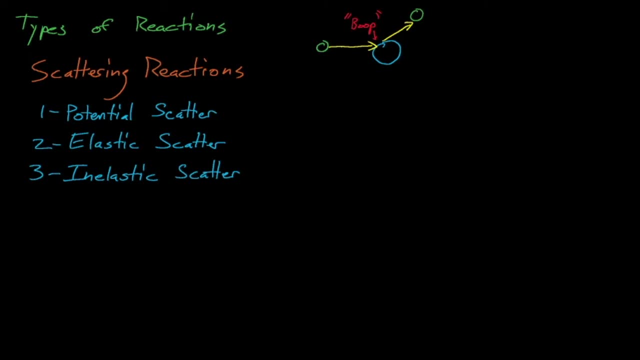 re-emitted. The neutron leaves the nucleus so quickly that it does not leave the nucleus in any kind of excited state, which means that kinetic energy is once again conserved between the target nucleus and the instant particle. During inelastic scattering, a neutron is 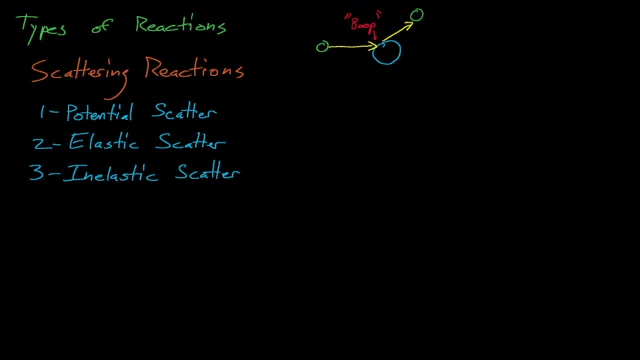 absorbed by the target nucleus before being re-emitted with less energy than it started with, which means that our neutron transfers enough energy to the target nucleus to leave it in an excited state. Eventually, this target nucleus will have to de-excite, which it often 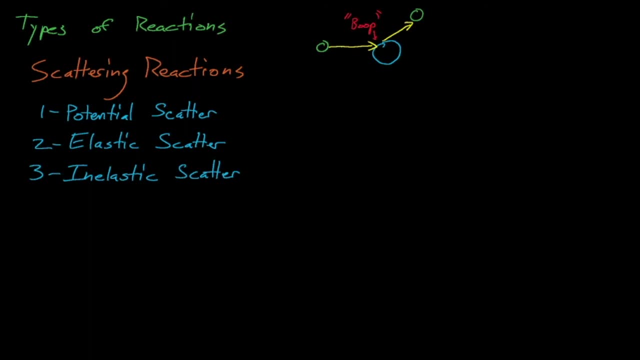 does by emitting a gamma ray. Because of this excitation, kinetic energy is not conserved during inelastic scattering and, in general, neutrons can lose a lot of kinetic energy during an elastic scattering event. An elastic scatter typically only occurs at higher energies. 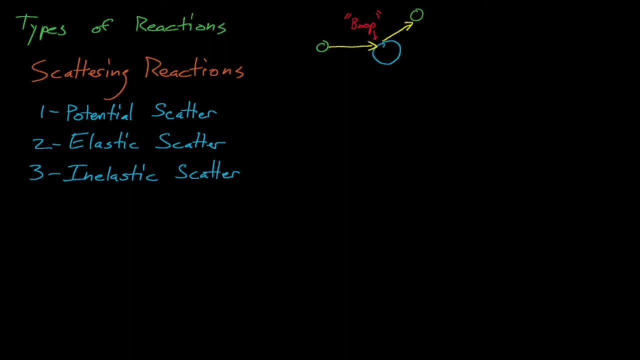 so above about 10 keV, which makes it an important mechanism affecting neutrons, slowing down and the neutron spectrum in fast reactors. Moving on to our other class of reactions, as the name suggests, absorption reactions involve a neutron that is absorbed after interacting. 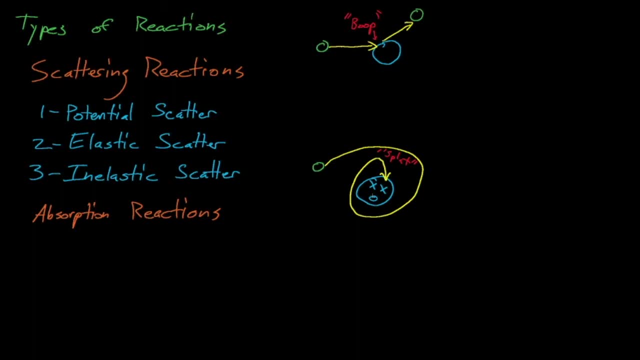 with some target nucleus. The target nucleus is left in an excited state due to the energy gained from the binding energy of the neutron, and the nucleus will have to emit some sort of particle to de-excite. During a radiative capture reaction, our target nucleus de-excites. 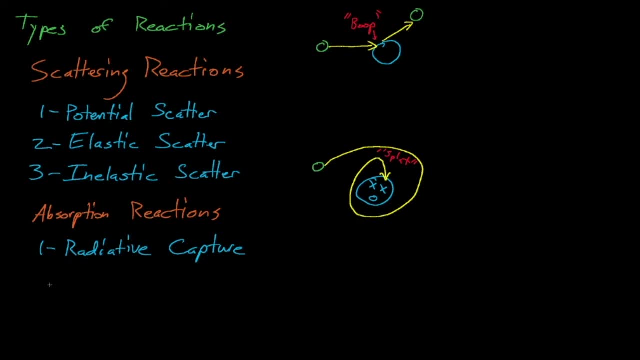 by emitting a gamma ray. This is a very common reaction that occurs during inelastic scattering, which may or may not cause other nuclei to transform into the Incredible Hulk. During N-P or N-alpha reactions, the nucleus de-excites by emitting a proton or an alpha particle. 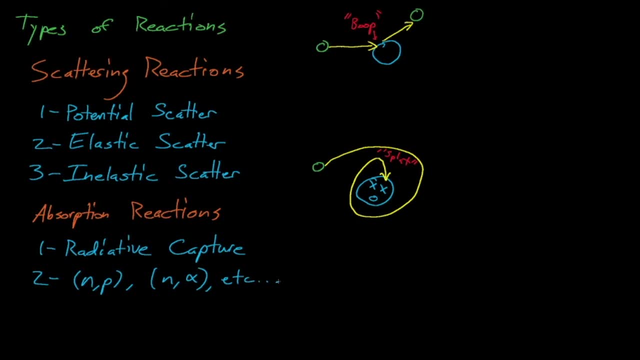 Excited nuclei can also de-excite by emitting a deuteron or a tritium particle or by emitting some even more exotic particles, but in general these reactions are less common than N-P or N-alpha reactions. Reactions can also de-excite by emitting multiple other neutrons, which results in